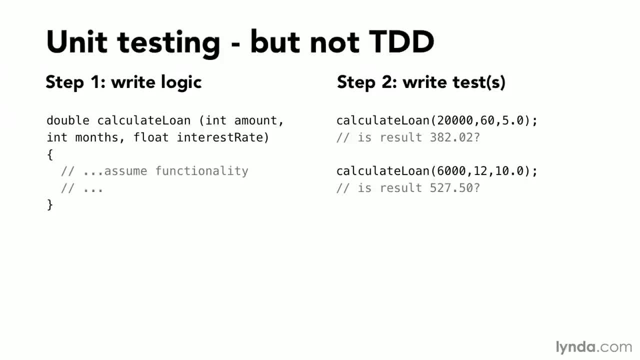 those results is what we expect And this is unit testing. We are testing and validating an individual method down to the individual unit in the code, But this is not test-driven development. Understand that TDD has the same two elements: a piece of application logic, a unit. 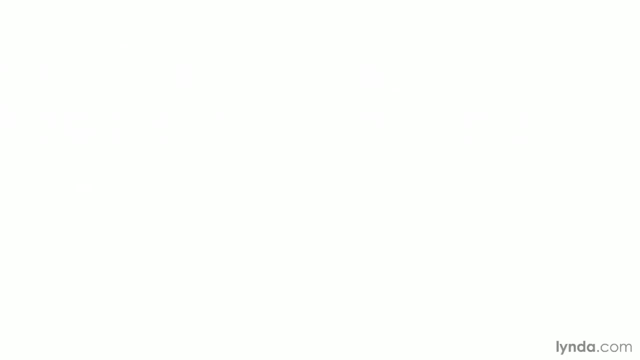 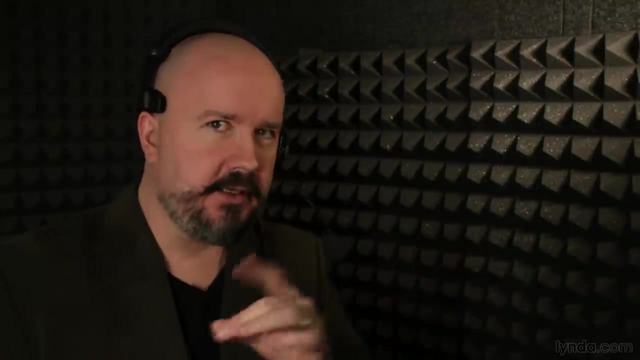 and a test, But it turns the process completely around. What test-driven development asks of us as developers is to write the test first before we write the application logic. That might sound counterintuitive, if not indeed impossible. But, Simon, I hear you say: 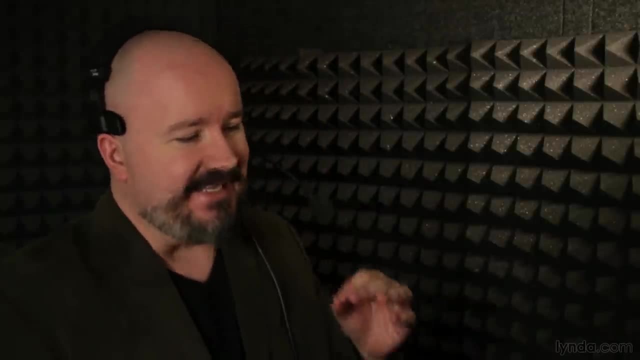 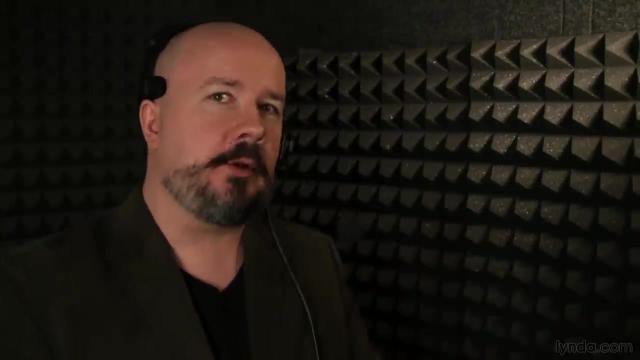 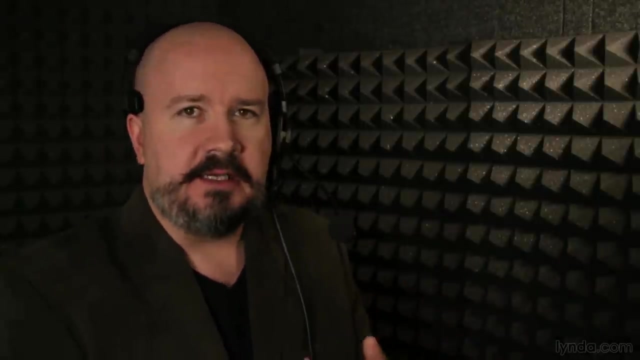 I can't exactly test a method I haven't written yet. Actually you can, And in test-driven development we do, And not just once or twice but all the time. We will write tests that attempt to instantiate an object Where we haven't written a class for that object yet. We will write tests that call a method that. 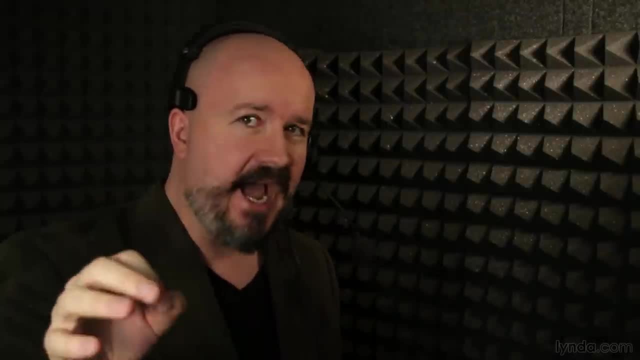 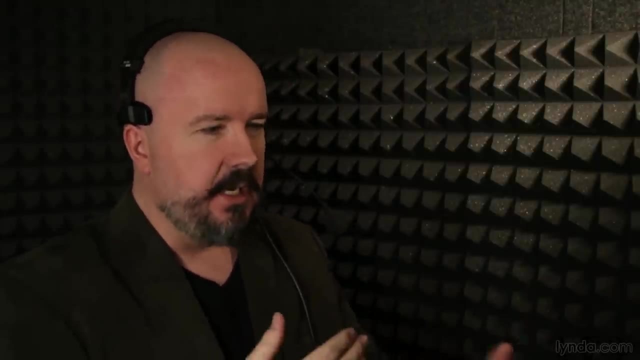 doesn't exist And we will run those tests. And the first time we run those tests they should fail. Depending on the language. they may not even compile, Or they might run and then tell us: well, I can't find this method, I can't find this class, But we want the test to fail Because after 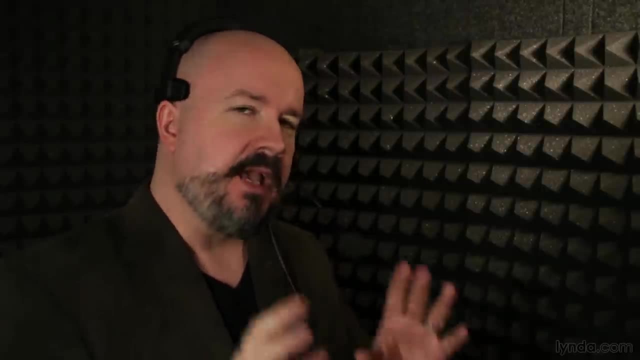 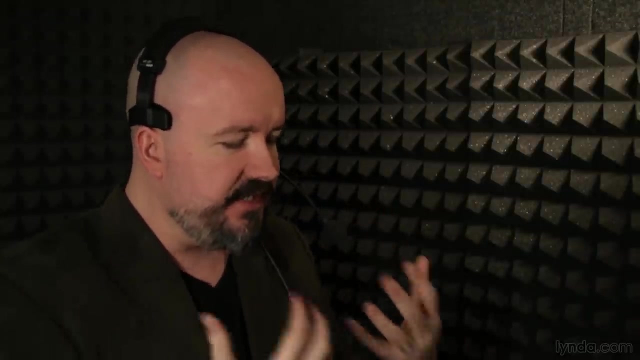 all. if it doesn't fail, we have some other kind of problem going on. And this is the fundamental first step of everyday test-driven development, The core distinction between doing TDD and not doing TDD- That before we write any new code. 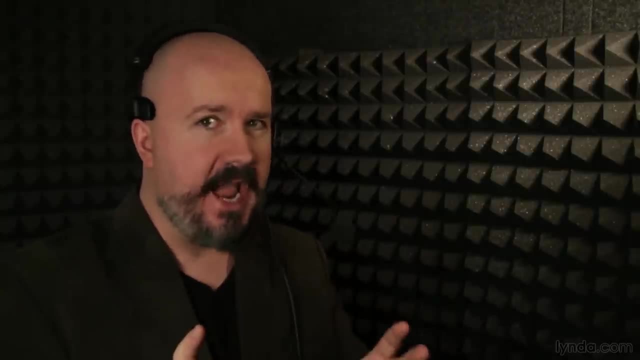 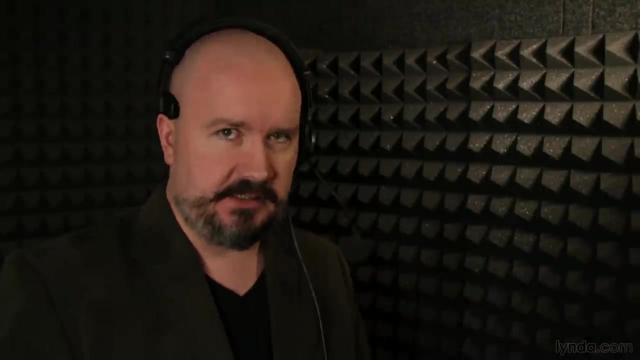 we first write a failing test And only after it fails do we write the application logic to pass that test And we write the minimum necessary code to just pass the test. One thing it immediately removes is the common situation where we create a new class or a new 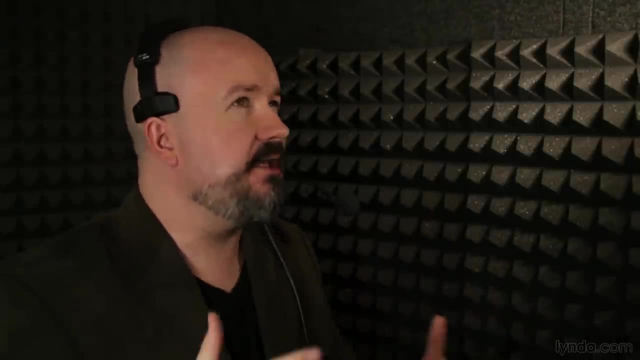 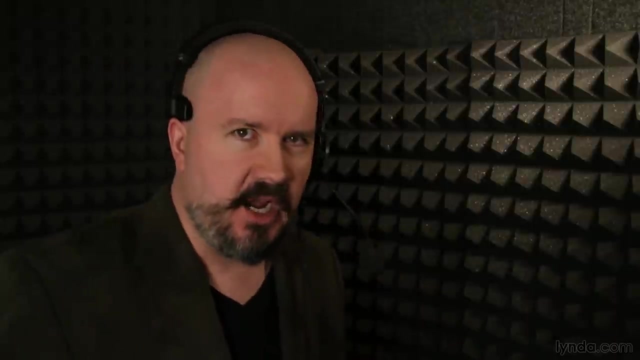 method and end up staring at a blank screen trying to juggle in our heads all the things this might need to do, And that's when we have a problem. And that's when we have a problem Today and tomorrow and in the future, all this speculative code that we're trying to come up. 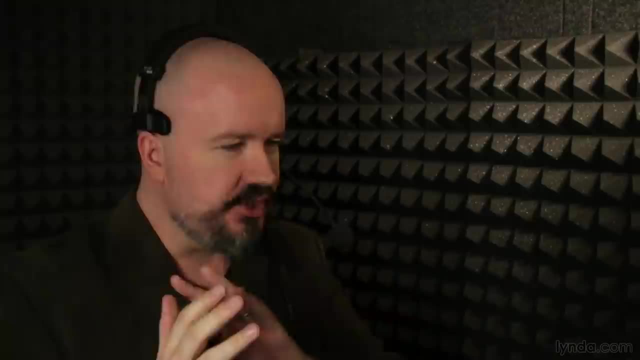 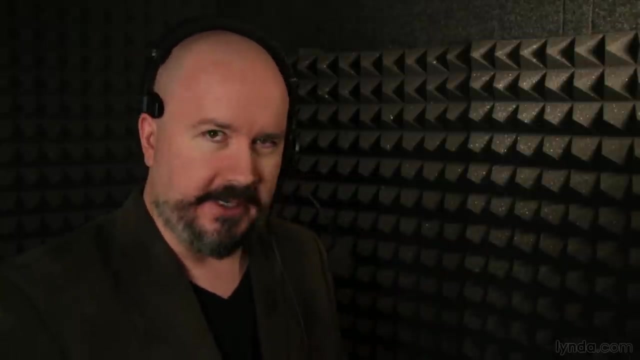 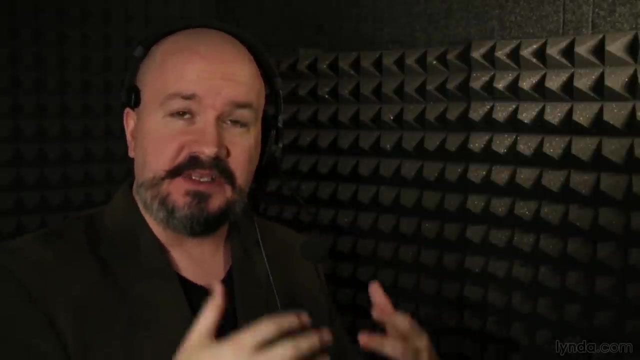 with. that is quicksand for every developer. No, just pass the test, this one test. it keeps us focused. This gives us clarity on exactly what we're doing at any one point. Don't do anything more than pass this small test, And this is what is meant by test-driven development. The tests: